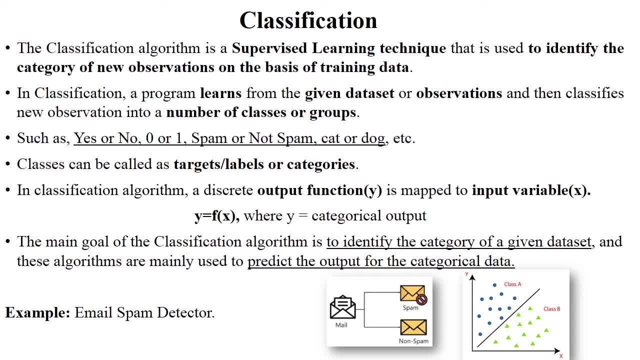 So for that purpose they use a particular words, For example, offers discounts, this kind of words they analyze and they identify the particular email is spam and not spam. So this is called as classification And see in this Below diagram, in this by below diagram, they generate the representation of classification. next, 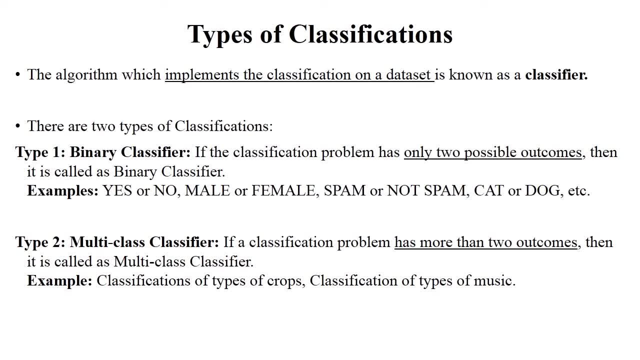 Okay, so the next point is types of classification. in machine learning There are two types of classification. One is binary classification and another one is multiclass classifier. So the algorithm which implements this classification in data set, This is known as classifier. 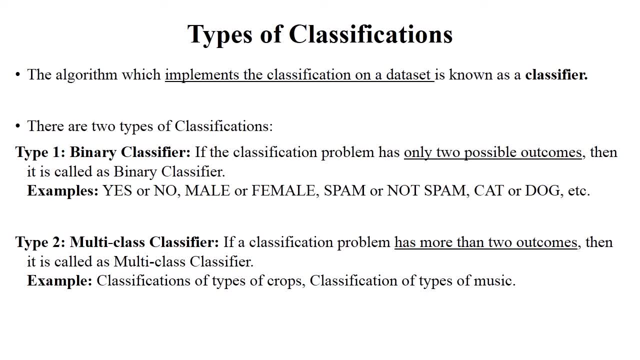 Okay, so first what is meant by binary classification? So binary classification, This means, if the particular classification problem having two possible outcomes, okay, only two possible outcomes. So this concept is called as binary classifier. For example, yes or no male, female, spam or not, spam then a cat or dog? 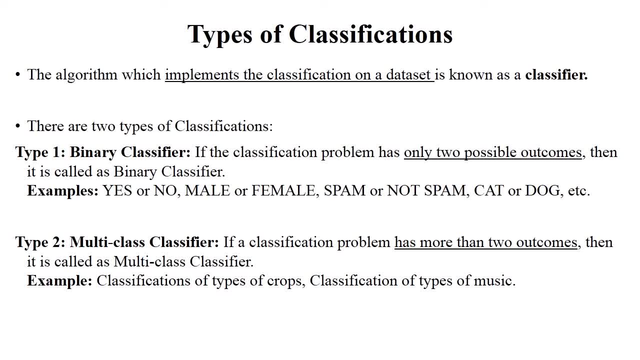 So this concept is called as binary classification. And the next type of classification is multiclass classifier. So multiclass classifier is obviously opposite of binary classifier, means if particular classification problem having more than two outcomes. So this concept is called as multiclass classification. 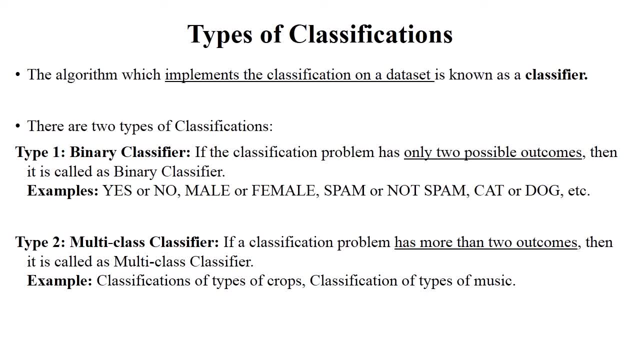 For example- see here the classification of types of crops- than classification of types of music. There are various types of music, various types of crops, Right, So these are the concept of multiclass classification and binary classifier. So what we learn? binary classifier means there are only two possible outcomes, and multiclass classifier means they have more than two possible outcomes. 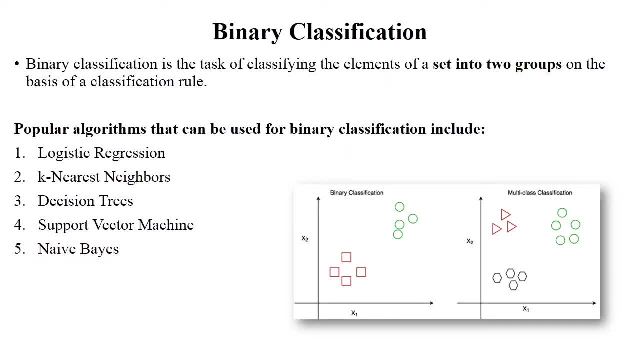 Right Next. So first we will learn about binary classification. Okay, So binary classification is a particular type of classification algorithm and they can generate a particular data set into the two groups. Miss. they classify the particular data into the two groups in two possible outcomes. 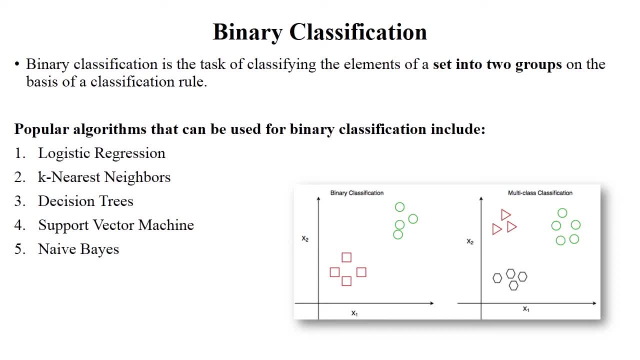 So see in this particular diagram, the first diagram, represent the binary classification. The particular shapes of data can be classified into the two parts. One is, for example, squared Data and another one is circular data. So this is called binary classification. and to implement this binary classification algorithm, 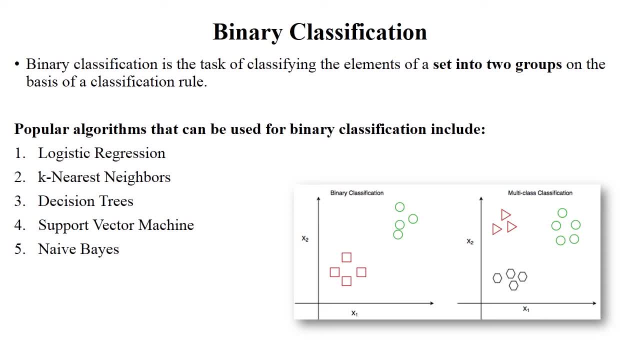 There are some popular algorithms are there, For example, logistic regression, K nearest neighbor decision, tree support vector machine and Navy bias. These are the some algorithms that is used for binary classification and we will learn all these algorithms one by one in next session. 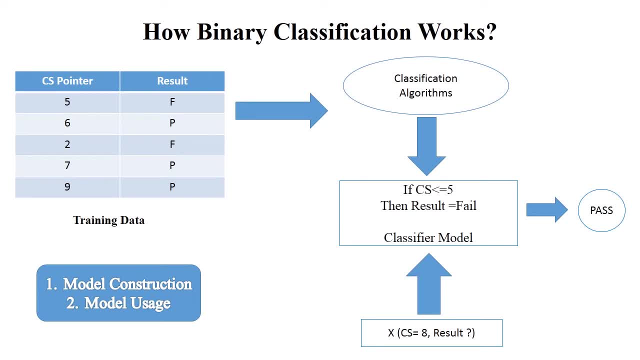 Okay, Okay. The next point is: see here How binary classification, Classification is work. See in this given example: there are two columns. One is suppose pointers, that is computer science pointer, and another column is result, Okay. So what is the concept of pointer? 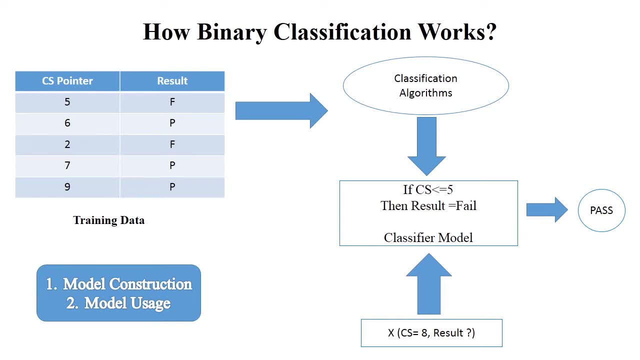 Suppose a particular student having the pointer for you, The result is: fail, Six pointer pass, two pointer fail, seven pointer pass and nine pointer pass. Okay, So what is the condition below five student having below five pointer, The particular Student is fail and more than five pointer. 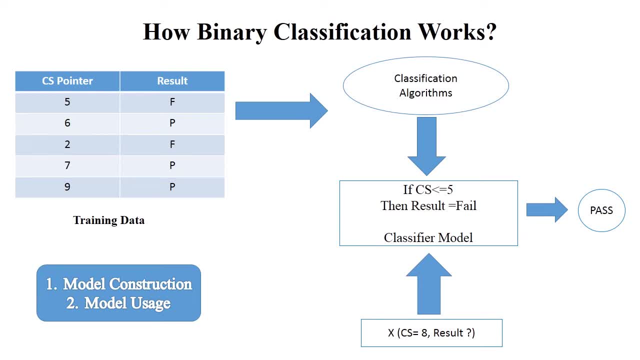 The particular student is pass Right, So suppose you need to classify this kind of data, So at that time this classification algorithm is work, So you need to apply the classification algorithm on this given data set. Okay Means you need to pass this data set as a input to the classification algorithm and you need to apply classification algorithm that have mentioned in previous slide. 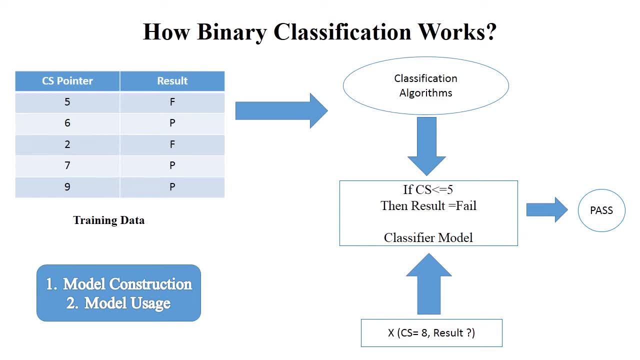 Okay, We will learn this classification algorithm Algorithm one by one in next session. So you need to apply this classification algorithm on this given training data and mention the condition. For example, see here: if the particular CS is less than equal to five, then result is fail. 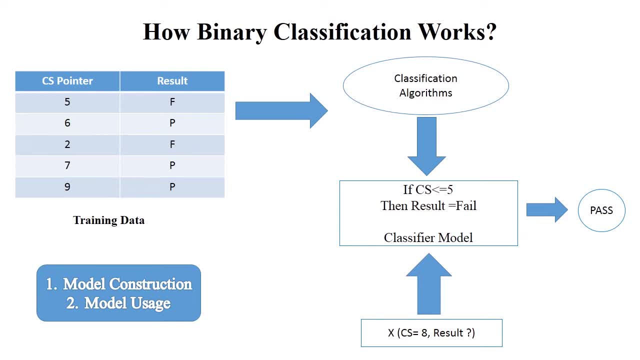 Otherwise, the particular student is pass. Okay, And this condition, this condition is called as classifier model- Okay, Classifier model represent a particular condition and you need to match this condition with your data set. So this work performed by the binary classification algorithm and in this way, you need to train the machine. 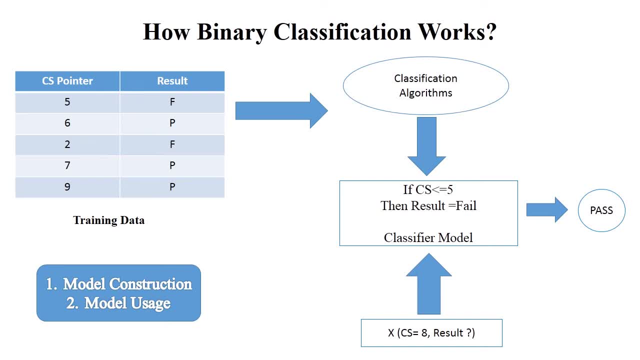 Okay, As per your training data, you train the machine and suppose after that, when you pass the particular data as an input to that particular machine- for example, you need to pass the CS pointer eight to the particular machine- So at that time you already train the machine. 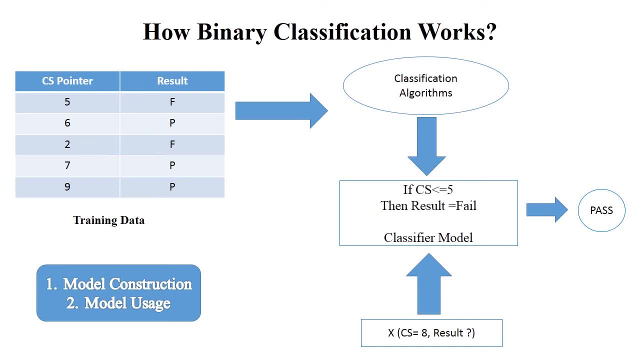 Right, So this eight pointer is checked with this particular condition. Machine check this eight pointer with this particular condition and generate the result whether the particular student is pass or fail. right, So you, you need to train the machine as per the classification algorithm or as per the algorithms, and after that you need to test the particular data with your machine. 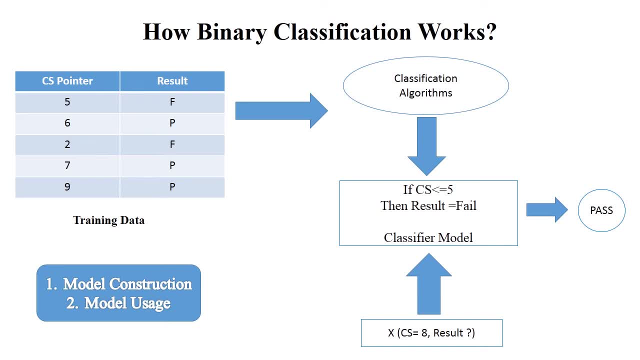 So this is a concept of binary classification work. So basically there are two steps. one is model construction, which is called as training data, as per training data Constructor model, and second one is model usage- means you need to test different data with this particular machine. online shopping website. 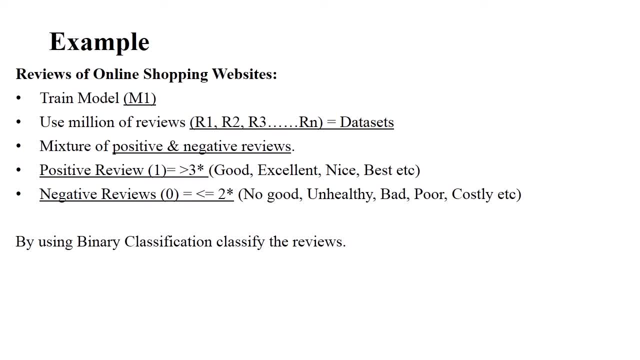 Okay, for example, suppose just consider that there is one model, This model is called as M1 and this is a training model. Okay, and in online shopping websites, there are multiple reviews from multiple users, right? So this, all the reviews are stored into the data set. 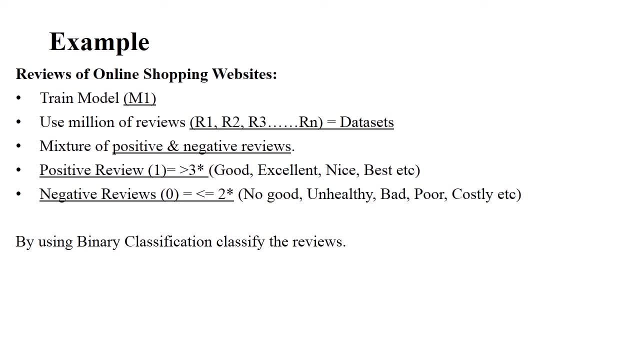 So just consider that there are R1, R2, R3 and multiple Up to Rn reviews are there, right? and these reviews are the mixture of positive reviews and negative reviews, right? So they classify the reviews as per their positive and negativeness. 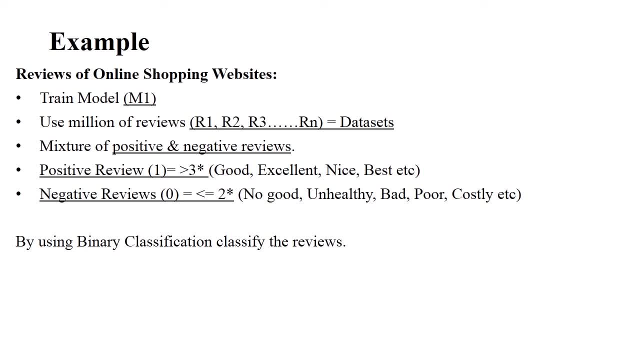 For example, positive review, positive review, which consider as one, and positive review means greater than three star rating. Okay and positive review contain the words like good, excellent, Nice, best, So this word include into the positive reviews, and negative reviews means that which consider. 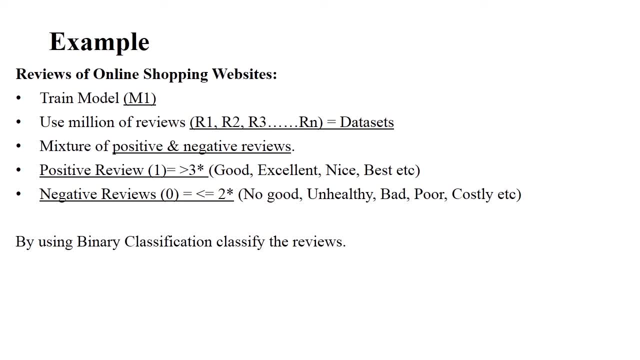 As 0, which is less than equal to 2 star, for example, no good, unhealthy, bad, poor, costly. So these words are include into the negative reviews. So in this way, online shopping website use classification algorithm to classify the reviews as per their rating, as per their words features. 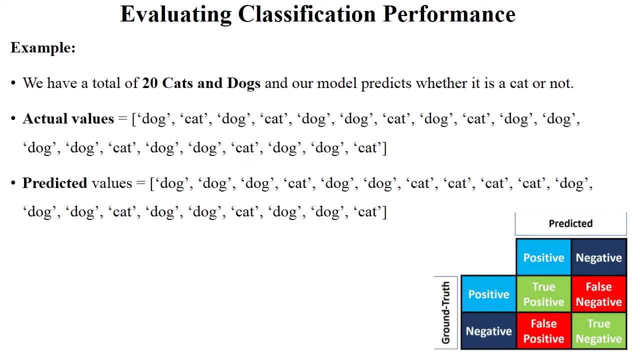 right next. Okay, Now the next point is evaluating classification. performance means how to evaluate classification algorithm. So for this purpose we use confusion Matrix thing. Okay, so see here in this example: suppose in our data set there are total 20 cats and dogs images. 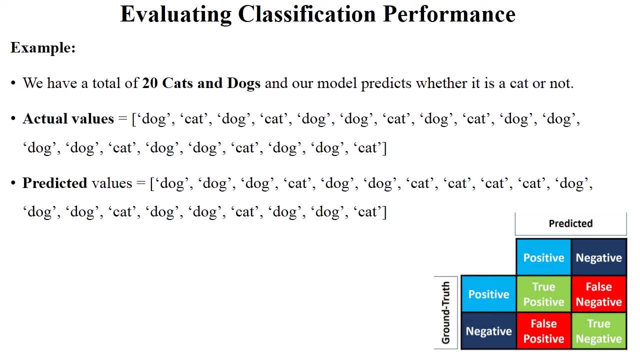 Okay and see there are two arrays are given, that is, actual value and predicted value. Suppose your actual value is dog and your predicted value is also a dog image. Okay, next one is: your actual value is cat and you are predicted that your the particular image is dog. 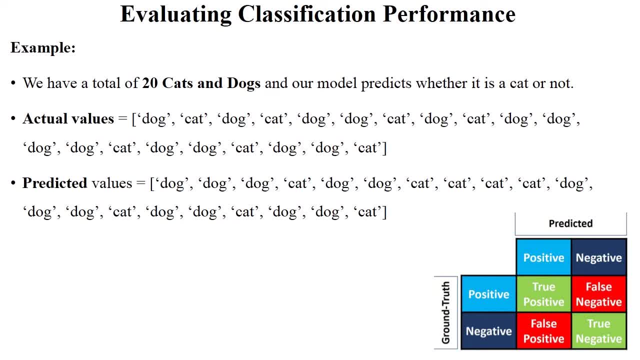 So in this There is actual value set and predicted value set is given. So in confusion Matrix there are total four results, which includes: see: in this diagram There is true positive, true negative, false positive and false negative, miss. There are two class, one is positive class and another one is negative class. 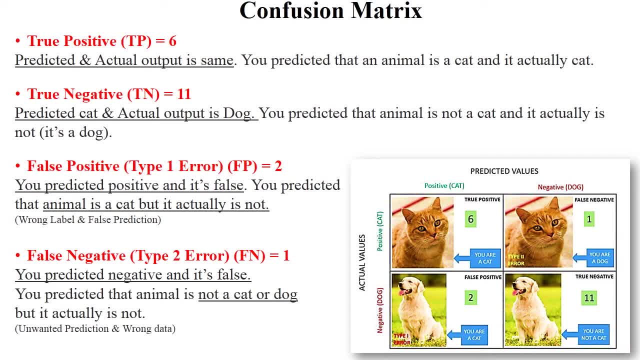 So let's see. Okay, so in confusion Matrix, the first one is true positive. What is mean by true positive? So true positive means your predicted data And your actual output data is same. This thing is called as true positive means your predicted that the particular animal is cat and your actual output is also cat. 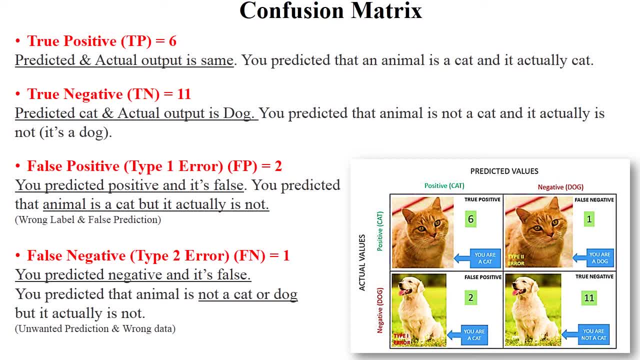 So this thing is called as true positive. see, in this diagram There are total six images are there in this given data set were perfectly match. The next one is a true negative. So true negative means suppose you are predicted that the particular image is cat, but your actual output is dog. 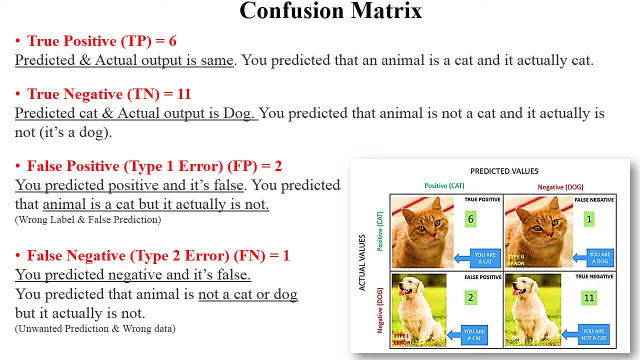 So there is a difference between predicted data and actual output data. So this thing is called as true. negative. in this image- See here- There are total 11 images. are there? 11 data are there which is true, negative? So next one is false, positive. 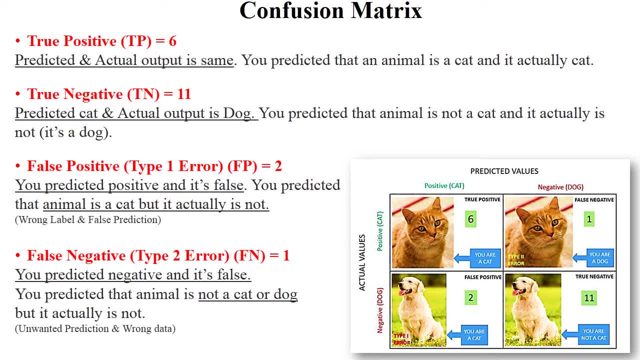 So false positive means you are predicted that positive and it's false means suppose you are predicted that the particular animal is cat but it is actually not a cat. in false positive there is wrong label And false prediction are there. see here in this diagram. in false positive: 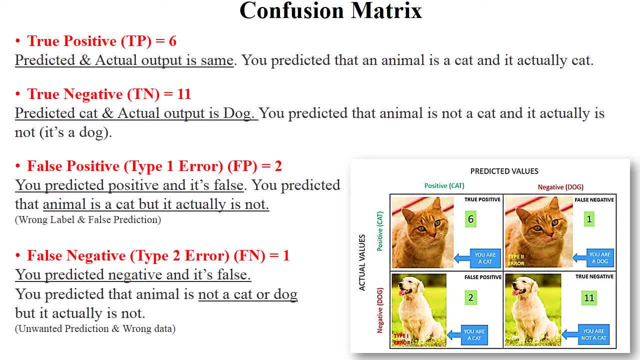 The particular level is you are cat, but image is for dog means there is a wrong level and false prediction is there. So this concept is called as false positive and this, this is also known as type 1 error. Next thing is false negative. So false negative means your predicted negative and it's false means your predicted that your animal is not a cat and not a dog.